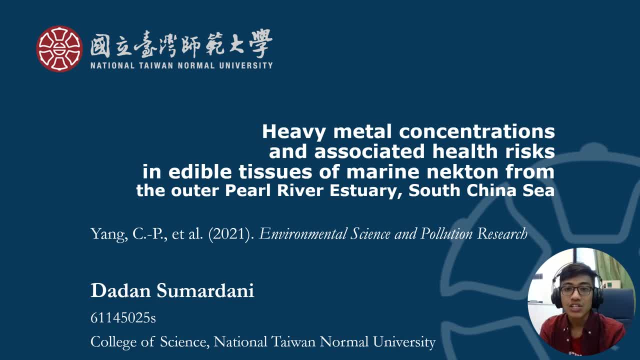 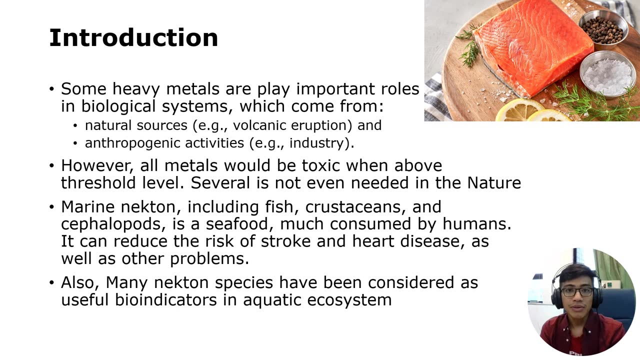 The title is Heavy Metal Concentration and Associated Health Risks in Edible Tissue of Marine Necton from the Outer Fur River Estuary. In introduction: some heavy metals apply important rules in biological systems which come from natural sources, for example from volcanic eruption rock. 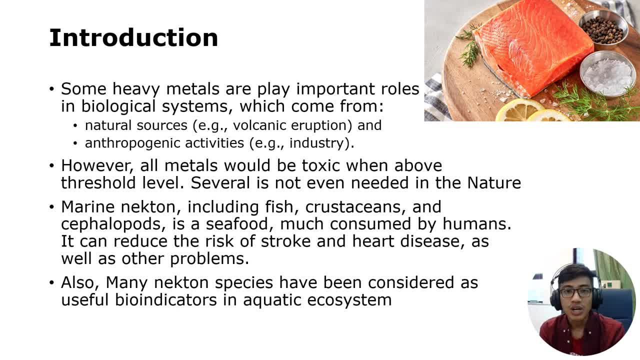 And in other hand it can be also coming from anthropogenic activity, for example industrial, for example human activity, sludge and other things. However, all metal will be toxic when above threshold level, Several is not even needed in the nature. 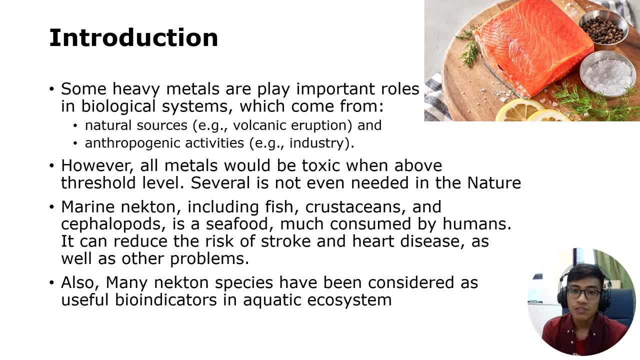 And then marine Necton, including fish, crustacean, and then cephalopod, is a seafood which much consumed by human. It can reduce the risk of stroke and heart disease as well as other problems. 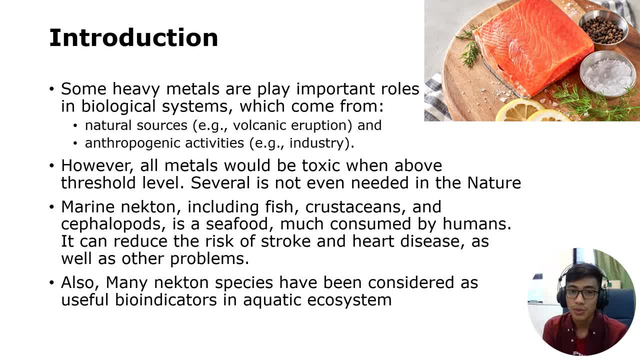 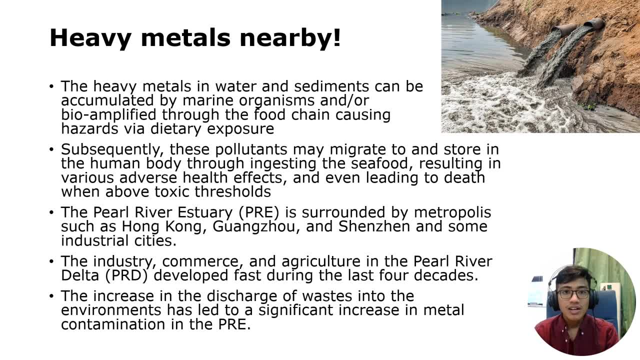 Also many Necton species has been considered as useful bio-indicator of aquatic ecosystem. So there are a lot of heavy metals nearby us, And then the heavy metal in the water and sediment can be accumulated by marine organism. 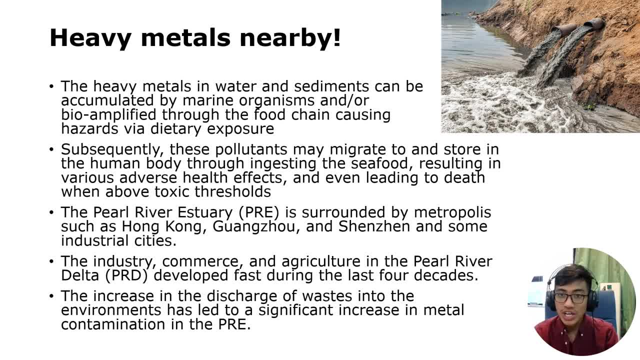 and or bio-amplified through the food chain, causing hazard via dietary exposure. Subsequently, this pollutant may migrate to and store in human body through ingesting the seafood, resulting in various adverse health effects such as impaired 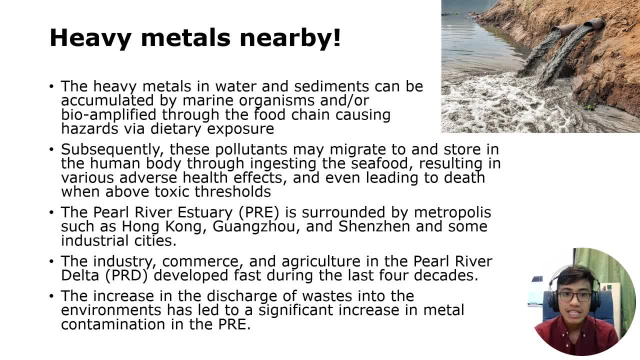 kidney function, poor reproductive capacity, liver damage, skin and bladder cancer and even leading to death when above toxic threshold. One of the case study in this research is the Perth river estuary is surrounded by metropolis such as. 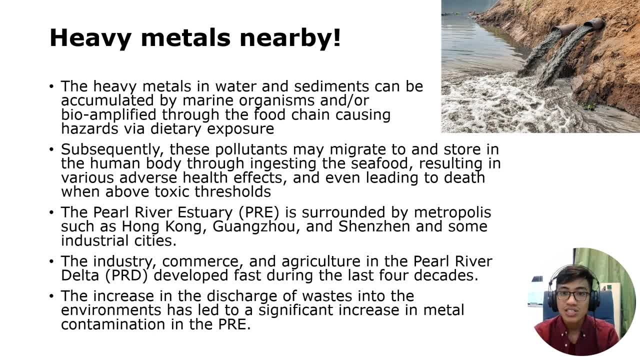 Hong Kong, Guangzhou and Shenzhen, and some industrial city like Dongguan, Zhongshan and Zhuhui in South China. The industry, commerce and agriculture in Perth river delta, PRD, developed for the last. 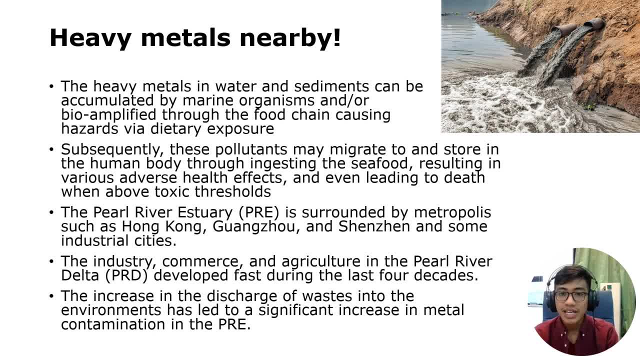 during the last four decades accompanying with the process reform and opening up in China. The increase is in charge. a lot of waste into the environment has lead to significant increase of water contamination in PRE. The objective of this. 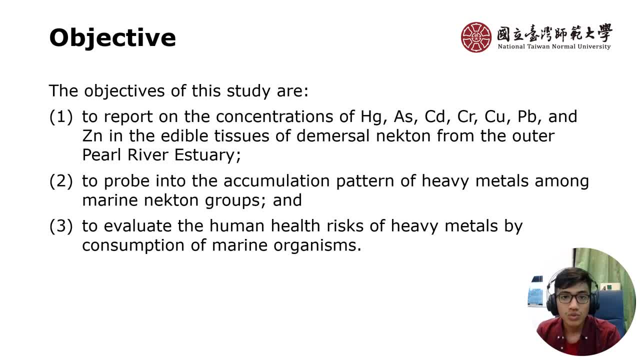 study include three things. number one, to report on the concentration of Hg, which is mercury, and then As, which is arsenic, and then Cd, which is cadmium, and then Cr, chromium, and then Cu, copper. 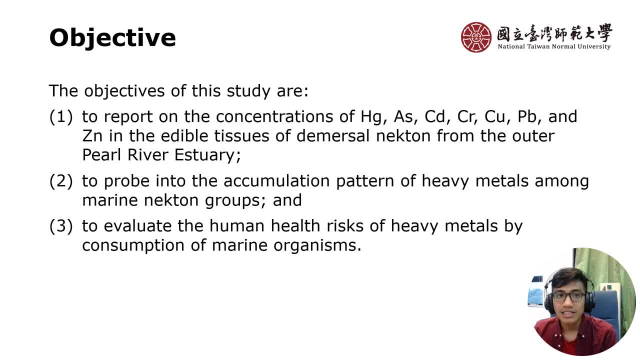 and then Pb, lead and Zn, which is zinc In the edible tissue of the myrtle nekton from the outdoor Perth river estuary. Number two, to prove, to probe into the accumulation pattern of heavy metal among marine. 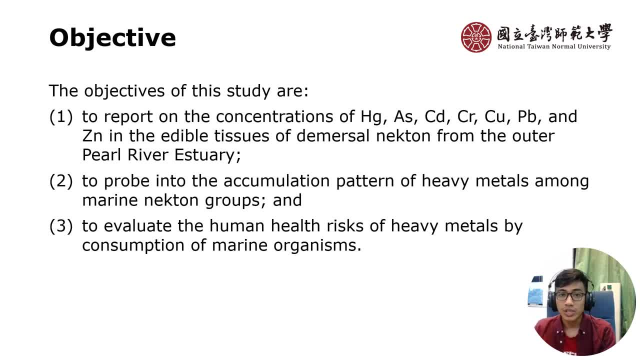 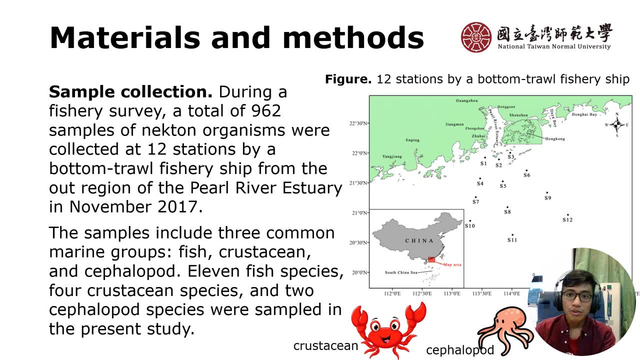 nekton group. and then the third will be to evaluate the human health risk of heavy metal by consumption of marine organism. Move to the next part will be material and method. So in sample collection we have several. 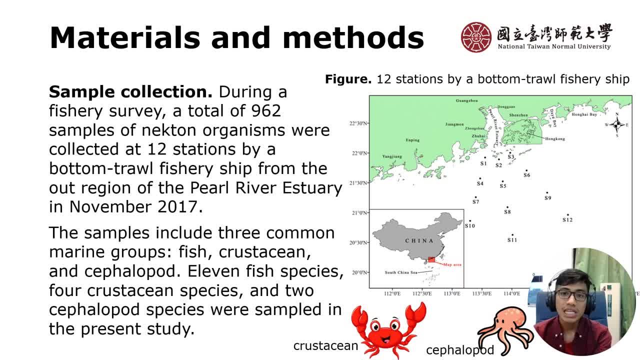 sample collection from the nekton nearby the place. So during a fishery survey a total of 962.. sample of nekton organism were collected at 12th station by a bottom trawl fishery ship from. 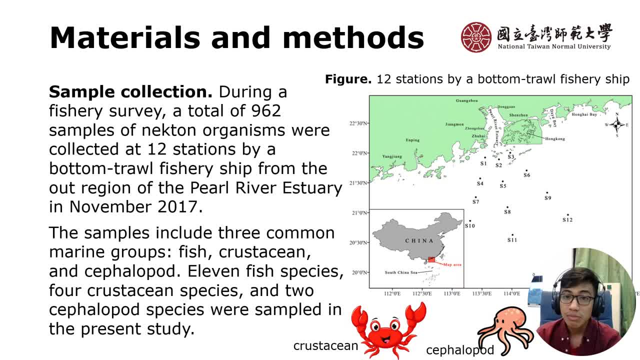 the out region of the Perth river estuary in November 2017.. As illustrated in figure one, The sample include 3 common marine group, which is fish, crustacean, and then cephalopod- 11 fish species. 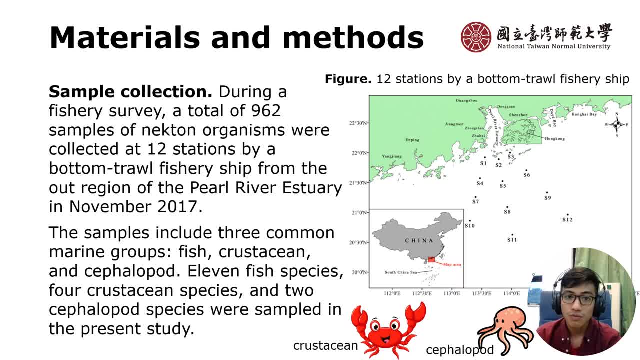 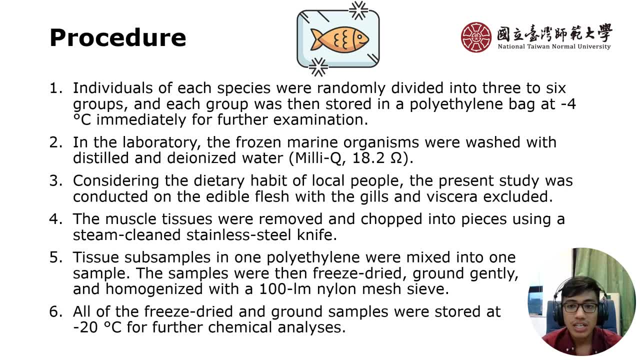 4 crustacean species and 2 cephalopod species were sampled in the present study. Each individual organism of each species were randomly divided into 3 to 6 groups, and then each group was then stored. 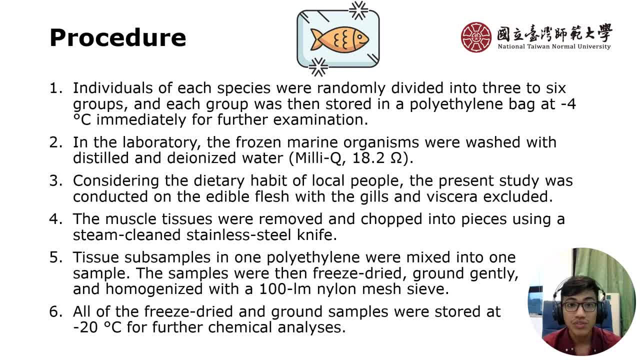 in polyethylene bag at minus 4°C. immediately for further examination In the laboratory. the frozen marine organism was washed with the distilled and ionized water. Then, considering the dietary habit of local people, the present study. 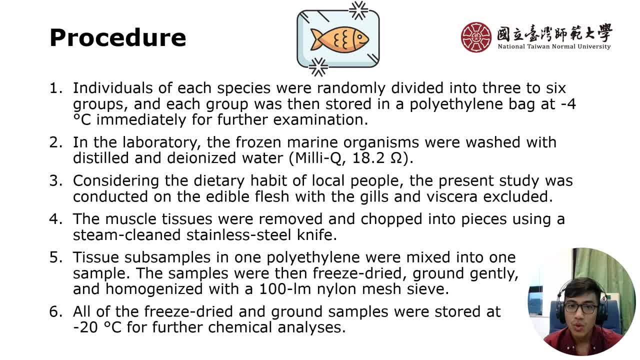 was conducted on the edible flesh, with the gill and fissura excluded. The muscle tissue were removed and chopped into fish using a thin, clean, stainless steel knife. Tissue subsampled in one. polyethylene were mixed into one. 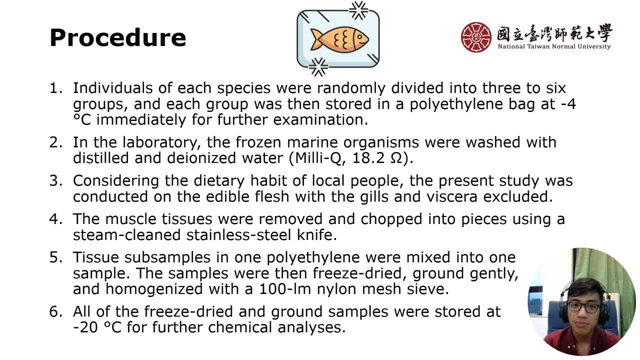 sample. The sample were then pre-dried gently and homogenized with 100 lm nylon mesh sieve. All the pre-dried and ground sample were then stored in minus 20°C for further chemical analysis. 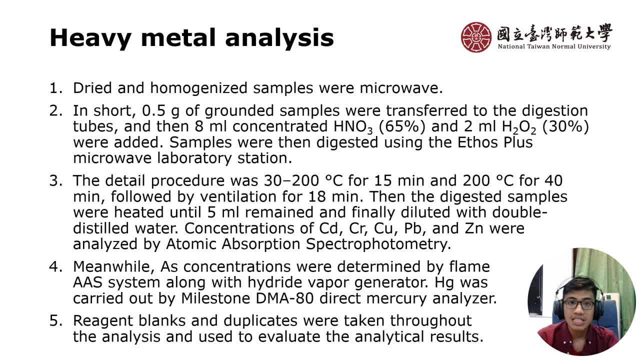 The next step is happy metal analysis. It started by dried and homogenized sample were microwaved. In short, 0.5.. gram of grounded sample were transferred to the digestion tube and then 8 mL concentrated. 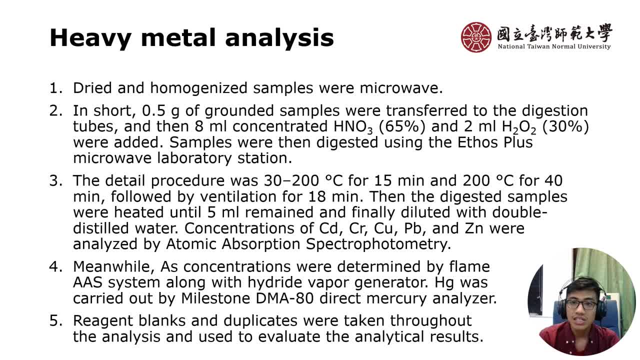 HNO3. and then 2 mL H2O2. were added. Sample were then digested using the Ethos Plus microwave laboratory station. The detailed procedure was 30 to 200°C for 15 minutes and then. 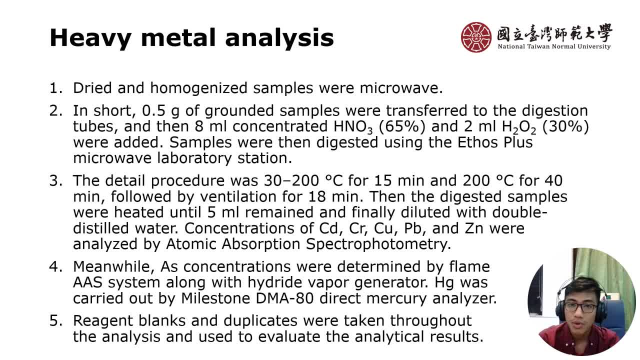 200°C for 40 minutes, Followed by ventilation for 18 minutes. Then the digested sample were heated until 5 mL remained, and finally diluted with double distilled water. Concentration of cadmium. 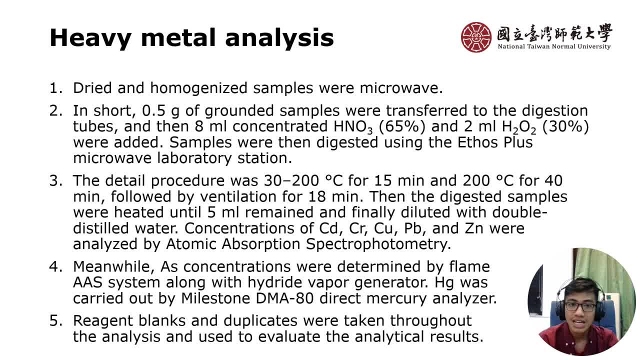 copper, lead and zinc were analyzed by Atomic Absorption spectrophotometry. Meanwhile, as concentration were determined by flame, AAS system, along with hydrate vapor generator, mercury were carried out by Milestone DMA-80.. 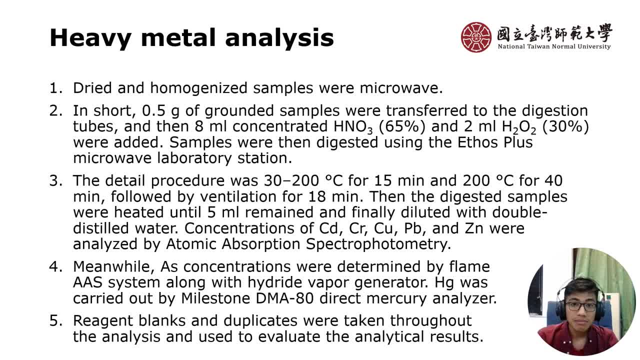 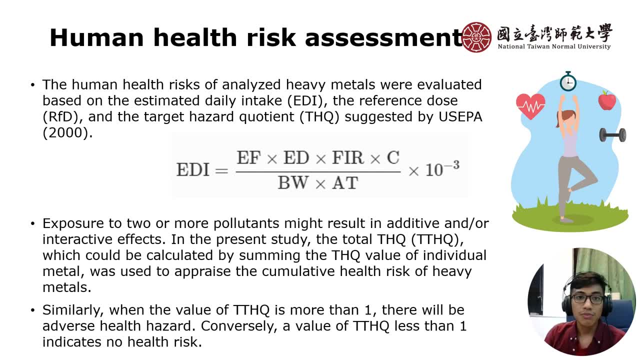 direct mercury analyzer Region. blank and duplicate were then, throughout the analysis, used to evaluate the analysis results. After finishing metal analysis, the next step will be human health risk assessment. So in this step, human health risk of. 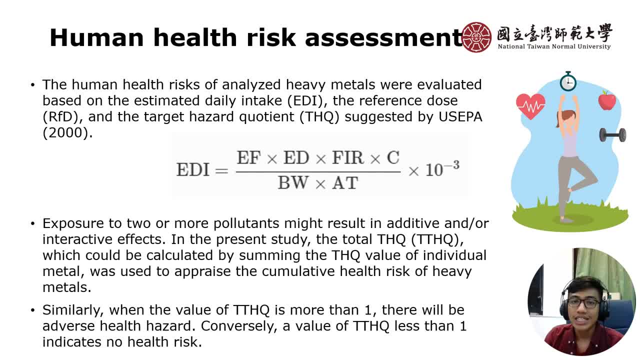 analyzed heavy metal were evaluated based on the estimated daily intake, EDI, and then the reference dose RFD and the target hazard question THQ and the formulation suggested by Yusefa in 2000.. So exposed. 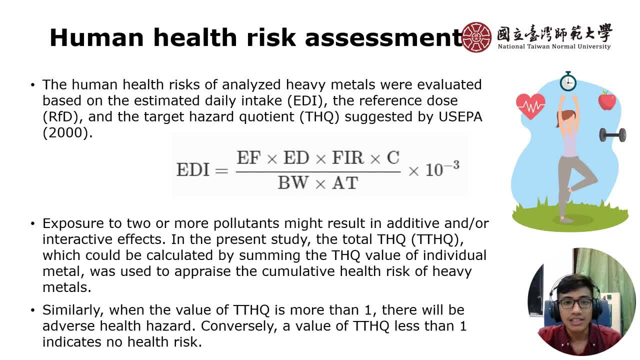 to two or more result in additive and or interactive effect. In the present study, the total THQ or TTHQ, which could be calculated by summing the THQ value of individual metal, was used to. 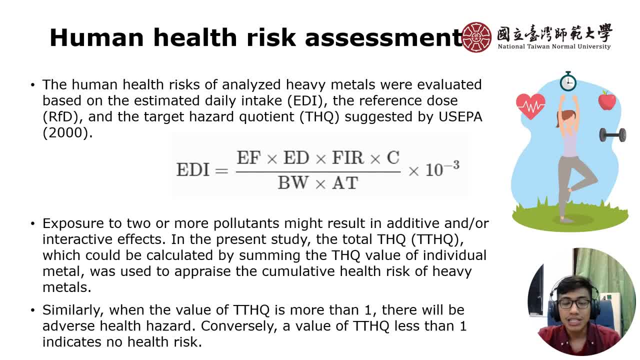 analyze the cumulative health risk of heavy metal. Similarly, when the value of TTHQ is more than one, there will be adverse health hazard. Conversely, a value of TTHQ less than one indicate no health risk. 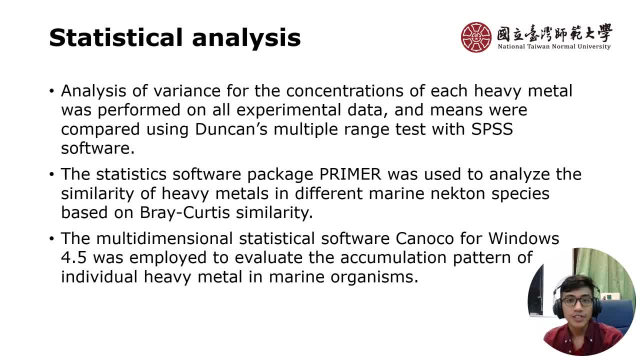 In statistical analysis of the result. analysis of variance for the concentration of each heavy metal was performed on all experimental data And mean were compared using Duncan multiple range test with SPSS software. The significant level was set up. 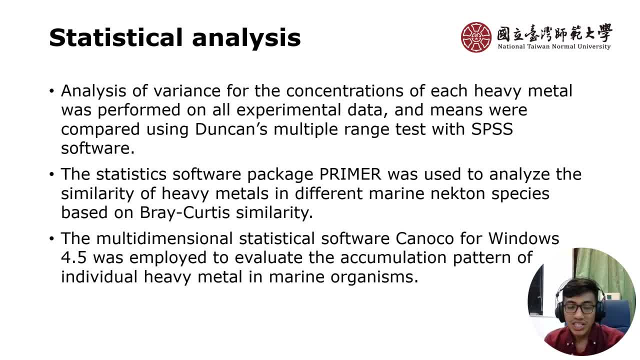 at V value less than 0.05.. The statistic software package primer was used to analyze the similarity of heavy metal in different marine necton species based on Bray-Carty similarity. The multidimensional statistical software Kanoko. 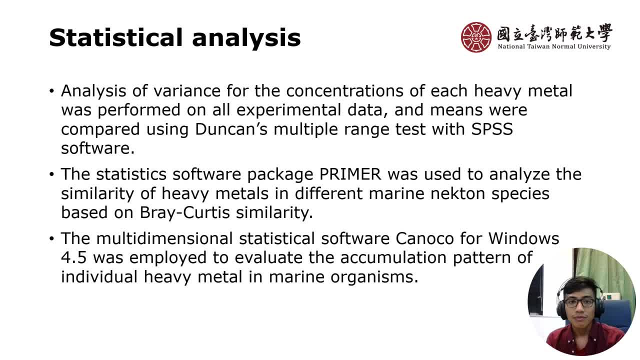 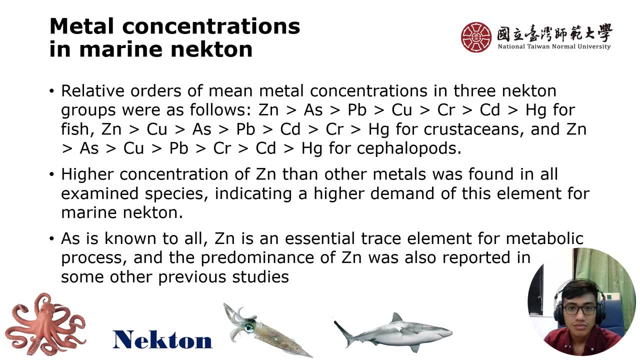 for Windows 4.5.. was employed to evaluate the accumulation pattern of individual heavy metal in marine organism. The next step will be result and discussion. The result on metal concentration in marine necton show some interesting. 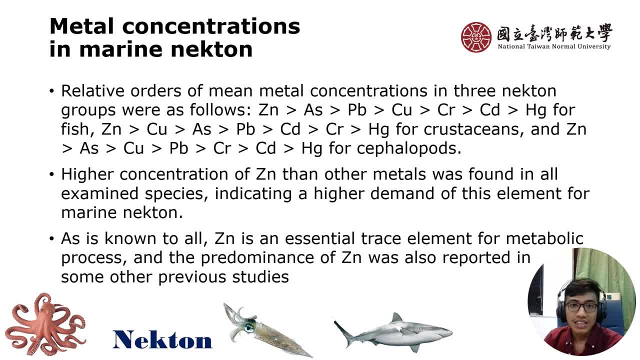 data. The first relative order of mean metal concentration in three necton group were as follow: For fish, zinc is bigger than arsenic and bigger than lead, bigger than copper, bigger than chromium, bigger than cadmium. 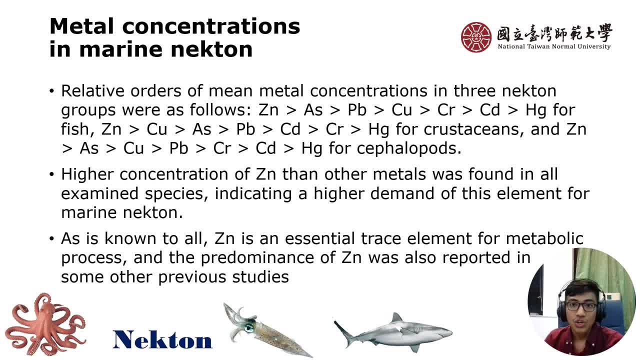 and bigger than mercury. And for crustacean zinc is bigger than copper, is bigger than arsenic, bigger than lead, bigger than cadmium and bigger than chromium and bigger than mercury. And lastly, for cephalopod. 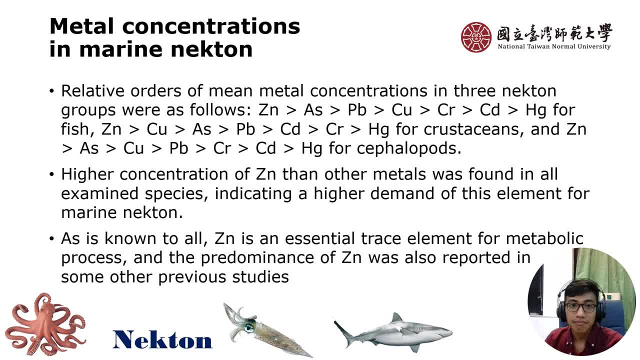 zinc is bigger than arsenic, bigger than copper, bigger than lead, bigger than chromium, bigger than cadmium and then bigger than mercury. Higher concentration of zinc than other metal was found in all examine species. 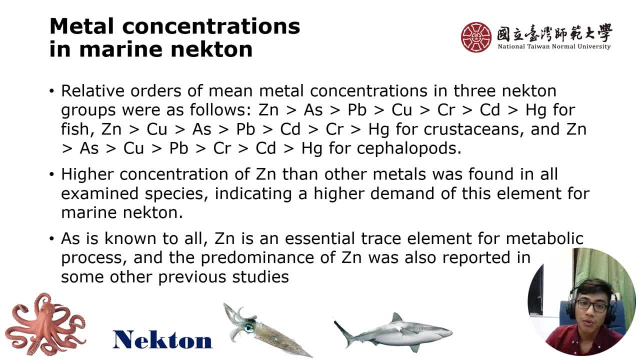 indicating a higher demand of this element for marine necton. As is known to all, zinc is an essential trace element for metabolic process and the predominant of zinc was also reported in soil. other previous study, One interesting: 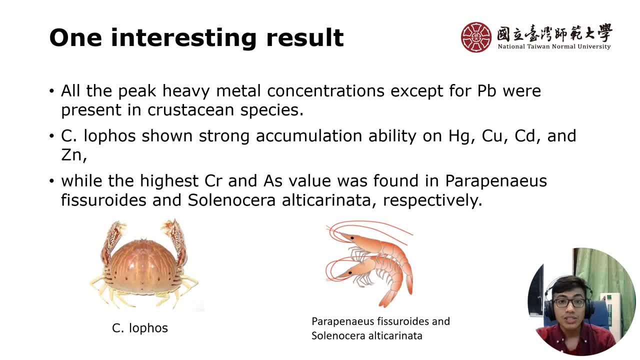 result in this study is all the peak heavy metal concentration, except for lead, were present in crustacean species, For example, lopos shows strong accumulation ability on mercury, copper, cadmium and zinc, while the highest 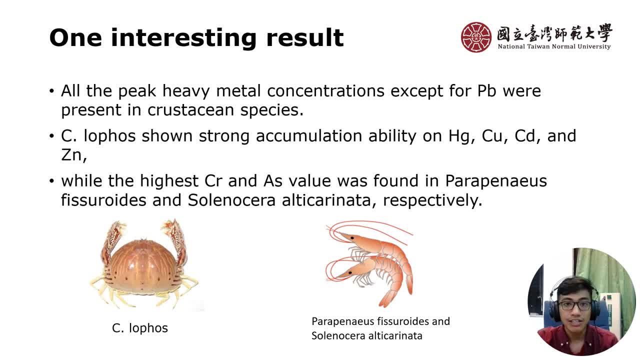 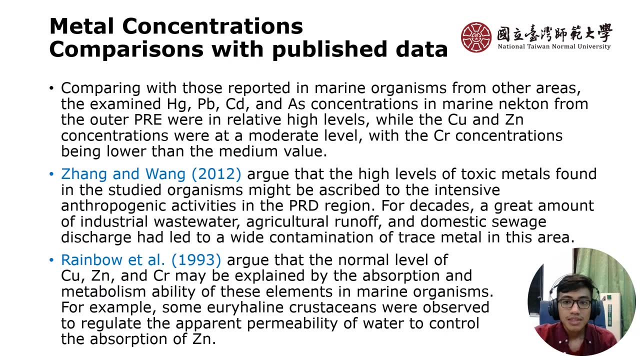 chromium and arsenic value was found in parapenaves, pisuroides and solone and soleno cera alti charinata respectively. The next part of result and discussion is metal concentration. 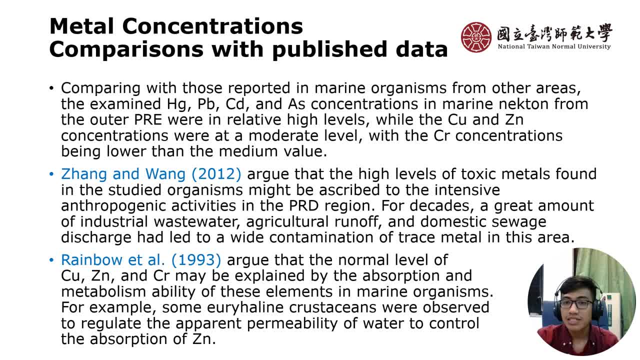 comparison with published data, so comparing with those reported in marine organism from other area. the examine mercury, lead, cadmium and arsenic concentration in marine necton from other PRE were in relative high level, while 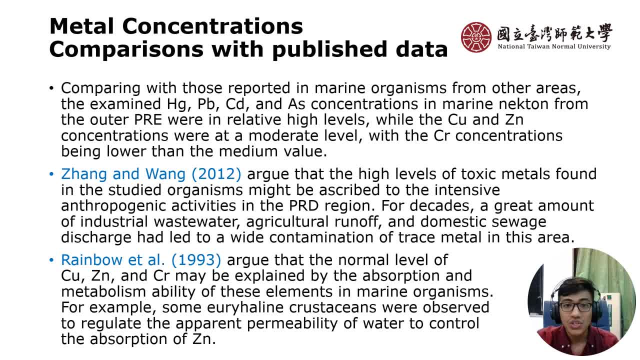 the copper and zinc concentration were at a moderate level, with chromium concentration being lower than the medium value, According to Zhang and Wang. he argued that the high level of toxic metal found in the study's organism might be. 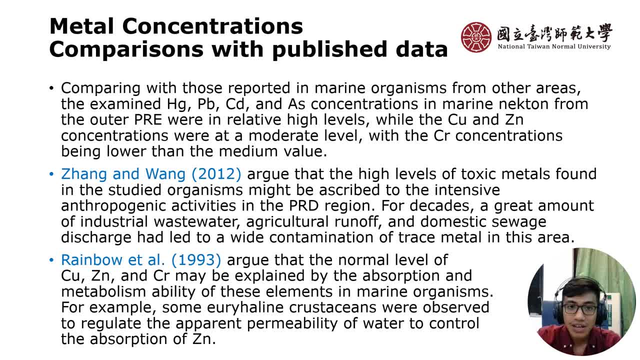 ascribed to the intensive anthropogenic activity in PRD region For Ticket. a great amount of individual wastewater, agricultural runoff and domestic sewage discharge had lead to a wide contamination of trash metal in this area, According to other study. 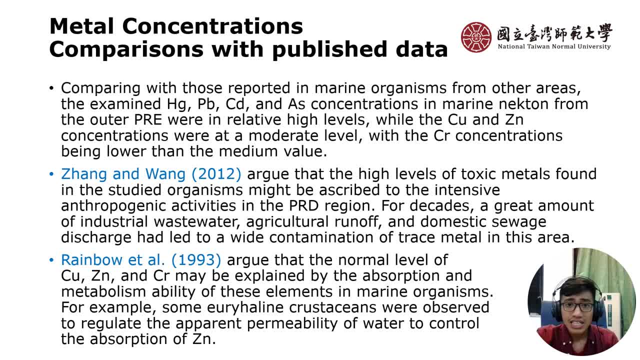 in 1993.. he argued that the normal level of copper, zinc and chromium may be explained by the absorption and metabolism ability of this element in marine organism. For example, some urihaline crustacean were observed. 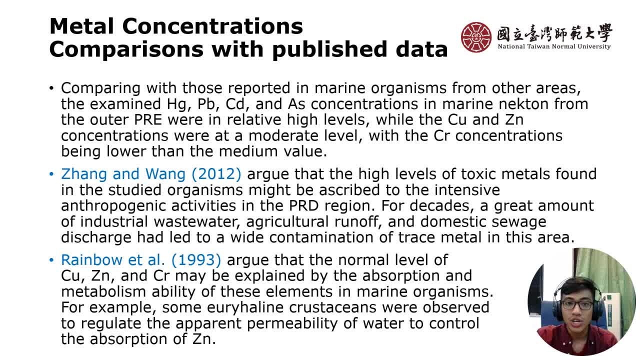 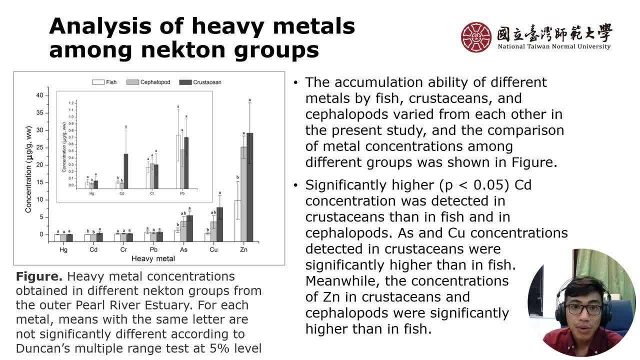 to regulate the apparent permeability of water. to control the absorption of zinc. This slide explaining the analysis of heavy metal among nekton group: Heavy metal concentration obtained in different nekton group from the outer for each metal. 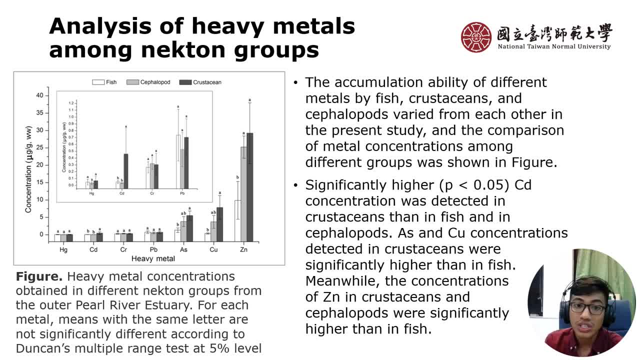 mean with the same layer, are not significantly different. according to Duncan multiple range test at 5% level, The accumulation ability of different metal in fish, crustacean and cephalopod varied from each other in the present. 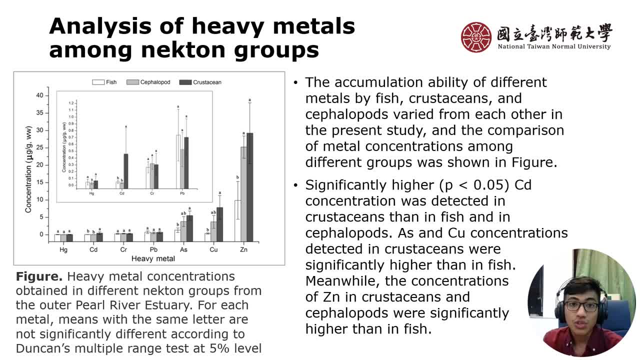 study and the comparison of metal concentration among different group was shown in figure. It is significantly higher cadmium concentration was detected in crustacean than in fish and in cephalopod. Arsenic and copper concentration detected in 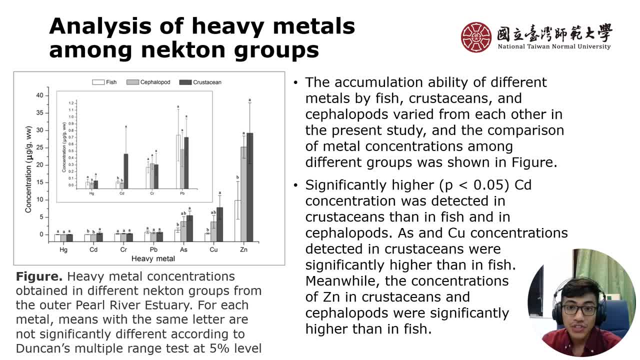 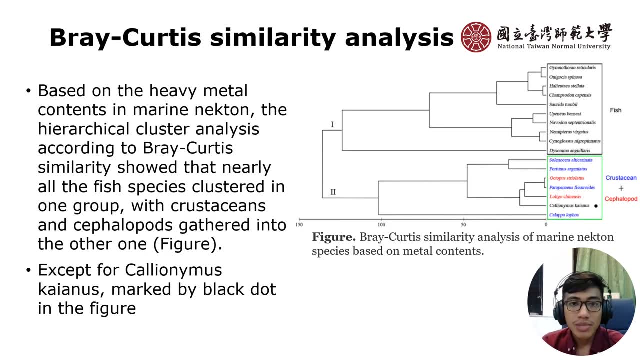 crustacean were significantly higher than in fish. Meanwhile, the concentration of zinc in crustacean and cephalopod were significantly higher than in fish. In addition, based on the heavy metal content in marine nekton, 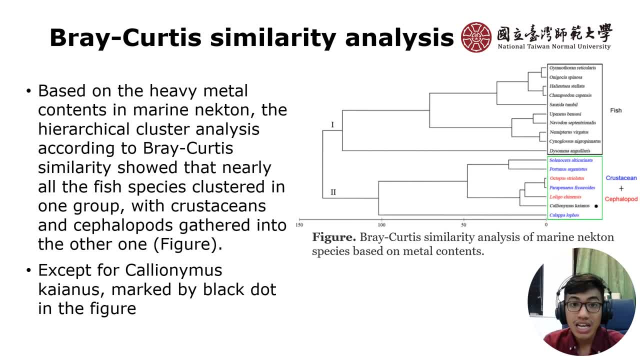 the hierarchical cluster analysis according to Bray-Curty similarity show that nearly all the fish species, except for Caleoneus Caleonimus Caeanus, marked by black dot in the figure cluster in one group. 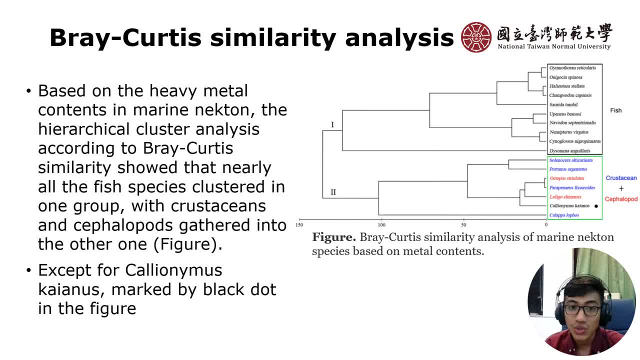 with crustacean and cephalopod gather into the other one. The figure is explaining Bray-Curty similarity analysis of marine nekton species based on metal content: All of the fish species except for C. 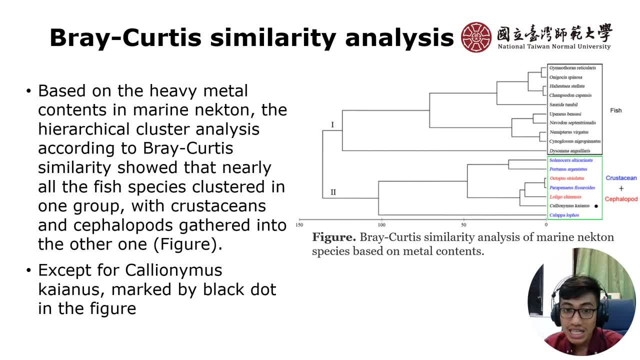 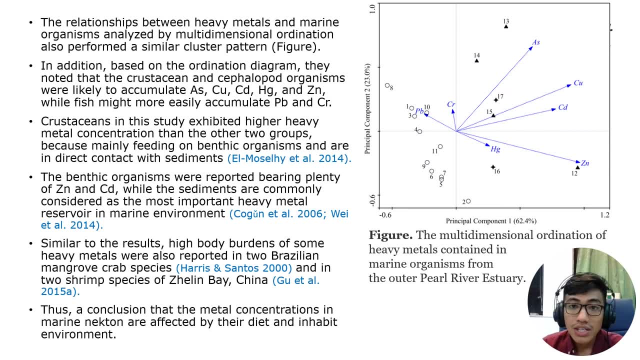 Caeanus group into cluster one, while the crustacean and cephalopod group into cluster two. The figure illustrate the multidimensional ordination of heavy metal contained in marine organism from the outer fur river estuary. Number indicate. 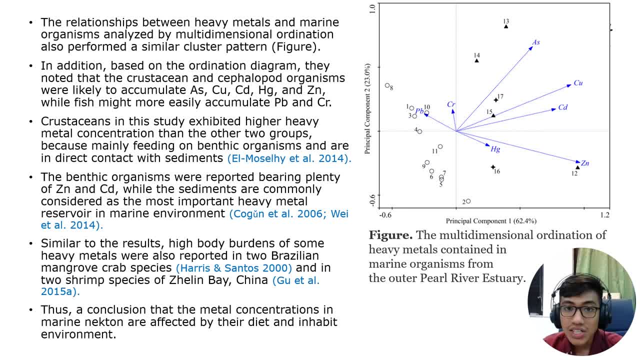 species name: Circle indicate fish, Triangle indicate crustacean and then star indicate cephalopod. Principle: component one and two explain the relationship between happy metal and marine organism. The relationship between happy metal and marine organism. 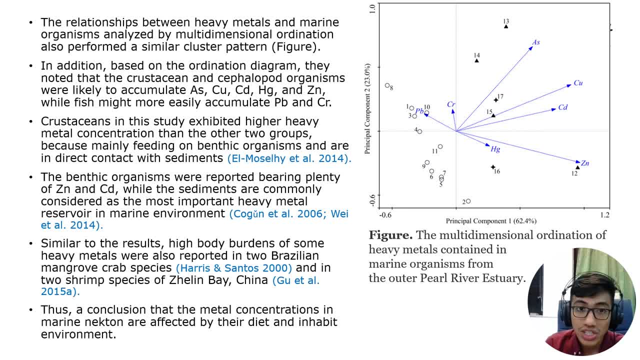 analyzed by multidimensional ordination also perform a similar cluster pattern. In addition, based on the ordination diagram, they note that the crustacean and cephalopod organism were likely to accumulate arsenic, copper, cadmium. 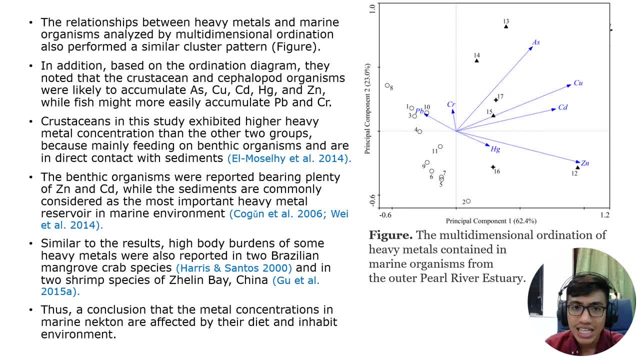 mercury and zinc. while fish might more easily accumulated lead and chromium, Generally crustacean in this study exhibit higher happy metal concentration than other two group because they mainly feed on benthic organism and are in direct contact with the 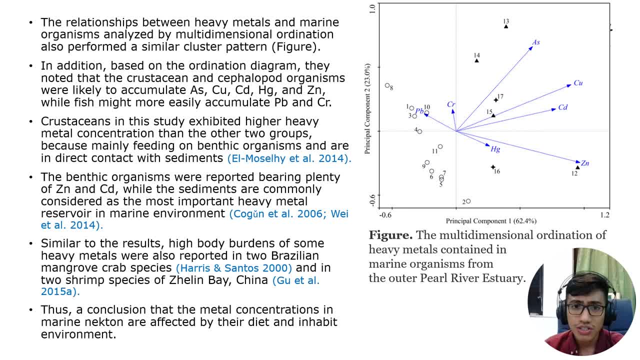 sediment, The benthic organism, such as Polychaetes, were reported bearing plenty of zinc and cadmium, while the sediment are commonly considered as the most important happy metal reservoir in marine environment. Similar to the result: high body. 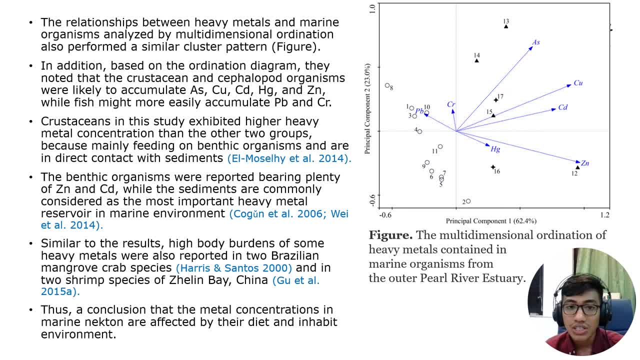 burden of some happy metal, for example zinc and copper, were also reported in two Brazilian mangrove crab species and in two shrimp species of Zeilin Bay in China. Thus a conclusion that the metal concentration in marine nectar are. 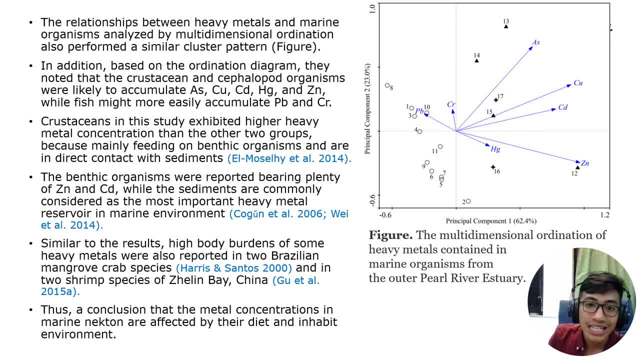 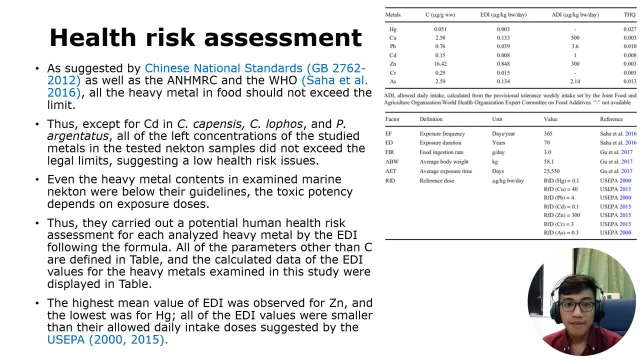 affected by their diet and inhabit environment. The next step will be human health risk assessment suggested by Chinese national standard, as well as the ANHMRC and WHO. All the happy metal in food should not exceed the limit as shown. 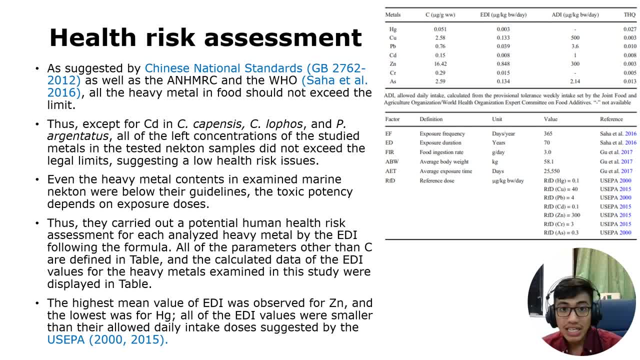 in the table. Thus, except for cadmium in sapendis, xylophos and P argentatus, all the left concentration of the study metal in the tested nectar sample did not exceed the legal limit suggesting a low. 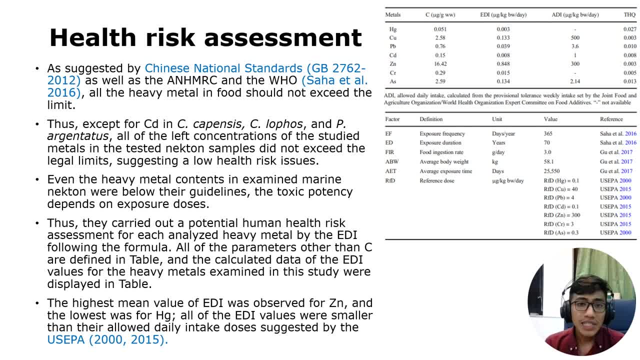 health risk issue. Even the happy metal content in the examined marine nectar were below their guideline. The toxic potency depend on exposure dose. Thus they carry out a potential human health risk assessment for each analyzed happy metal by. 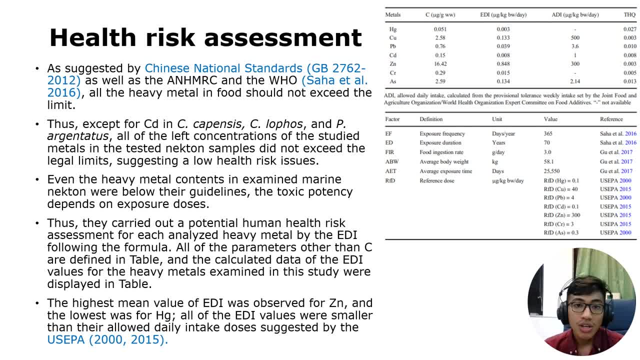 the EDI following the formula. All the parameters other than C are defined in table And the calculated data on EDI value for the happy metal examined in the study were displayed also in the table. The higher mean. 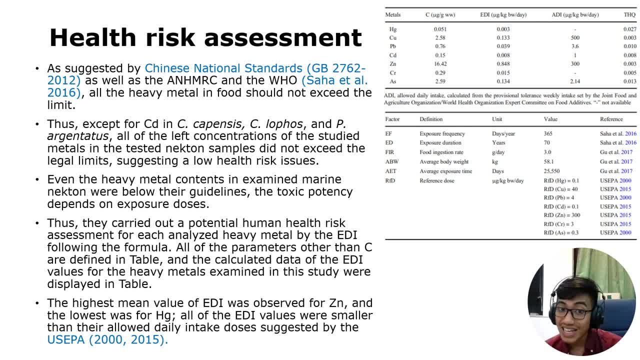 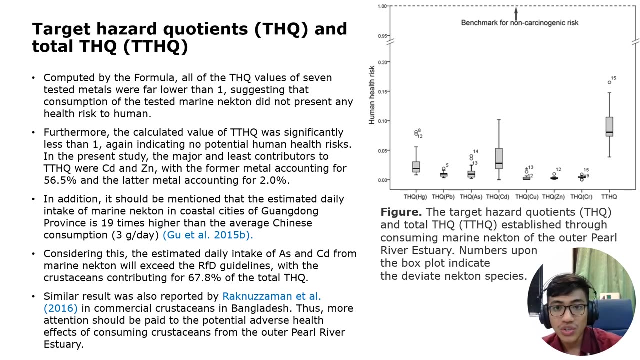 value of EDE was observed for zinc And the lowest was for mercury. All the EDI value were smaller than their low daily intake dose suggested by the USEPA. The figure illustrates the target hazard questions. 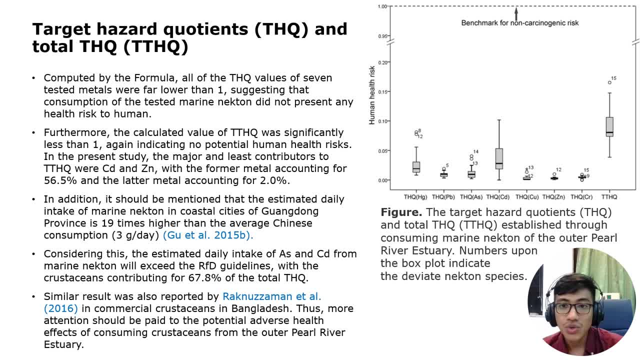 and total THQ established through consuming marine nectar of the Thir River. Asteroid Number given on the box plot indicate the deviation nectar species following the table in 50th slide, Computed by the formula all the. 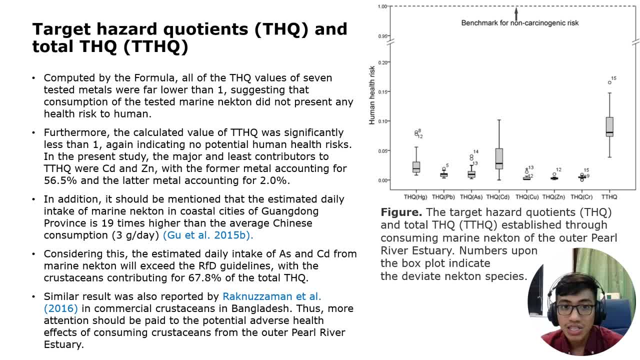 THQ value of 7 test metals were far lower than 1. Which suggesting that consuming of the tested marine nectar did not present any health risk to human. Furthermore, the calculated value of TTHQ were significantly. 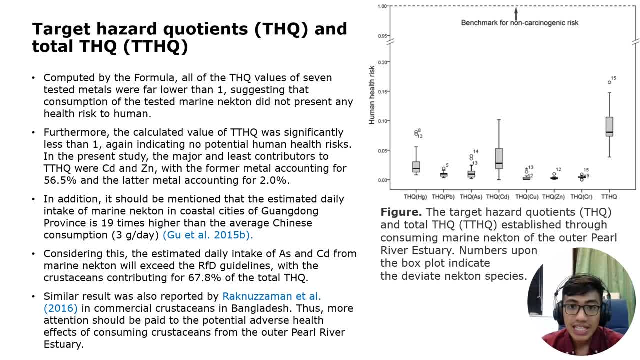 less than 1.. Again indicating no potential human health risk. In the present study, the major and least contribution to TTHQ were cadmium and zinc, With the former metal accounting for 56% and the later metal. 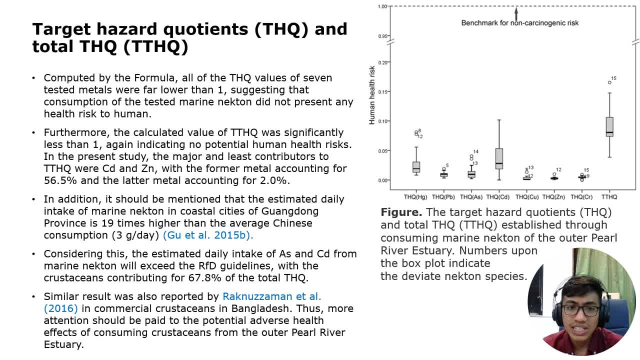 accounting for 2%. In addition, it should be mentioned that the estimated daily intake of marine nectar in coastal city of Guangdong province is 19. times higher than the average Chinese consumption. Considering this, the estimated daily. 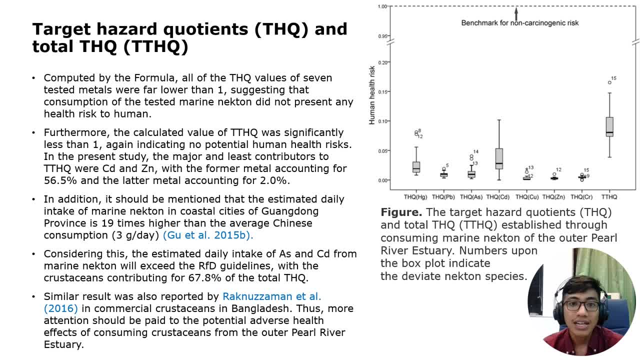 intake of arsenic and cadmium from marine nectar will exceed the RFD guideline, with the crustacean contributing for 67% of the total TTHQ. Similar finding was also reported by Ragh Nuz Zaman. 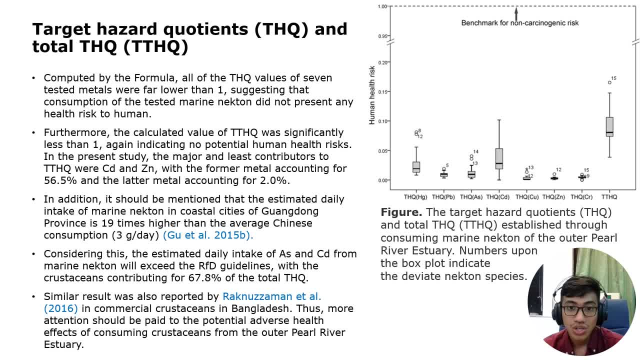 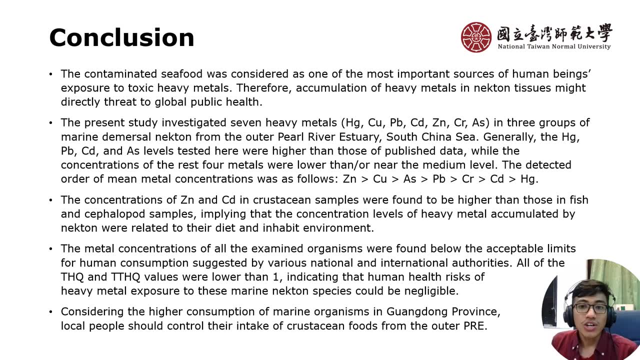 in a commercial crustacean in Bangladesh shows more attention should be paid to the potential adverse health effect on consuming crustacean from the outer third river estuary. Finally, the conclusion of the article: The contaminated. 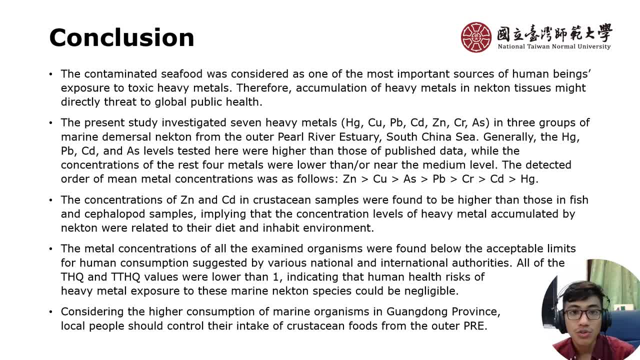 seafood was considered as the most important sources of human being exposure to toxic heavy metal. Therefore, accumulation of heavy metal in nekton tissue might directly threat to global public health. The present study investigates 7 heavy metal. 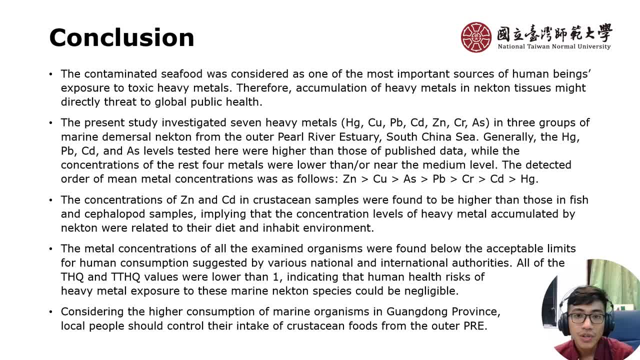 including mercury, copper, lead, cadmium, zinc, chromium and arsenic. in 3 group of marine demersal nekton from the outer third river estuary in South China Sea, Generally the mercury lead. 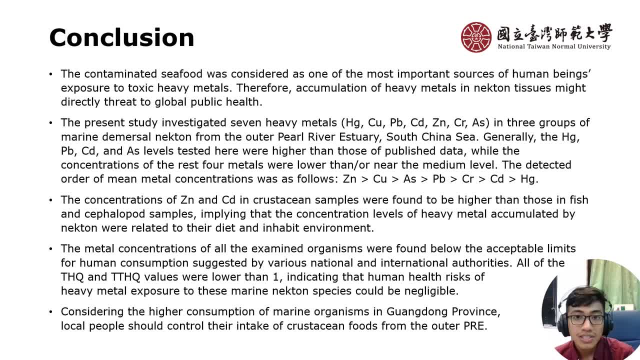 cadmium and arsenic level test here were higher than those of published data, While the concentration of the rest for metal were lower than or near the medium level. The detected order of mean metal concentration was as follow: Zinc is. 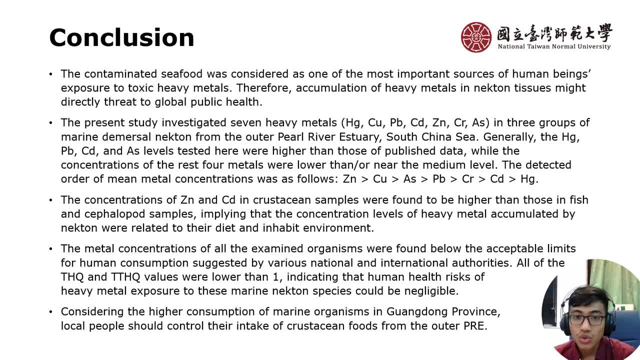 is bigger than copper, bigger than arsenic, bigger than lead, bigger than chromium, bigger than cadmium and bigger than mercury. And then the concentration of zinc and cadmium in crustacean sample were found to be higher. 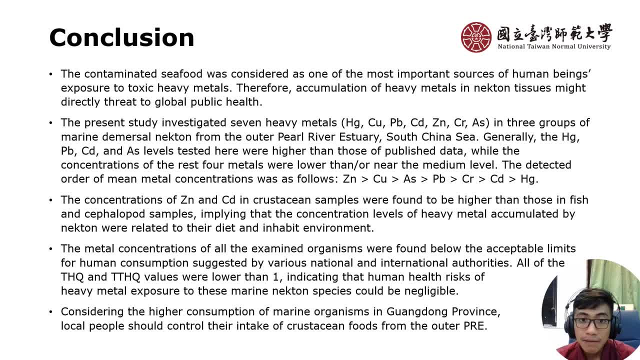 than those in fish and cephalopod sample, Implying that the concentration level of heavy metal accumulated by nekton were related to their diet and inhabitant environment, And then the metal concentration of all the examined. 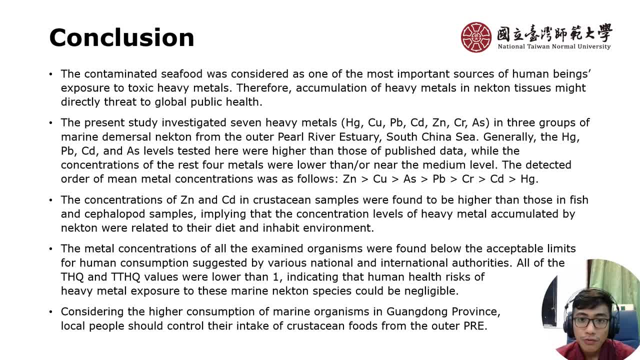 organisms were found below the acceptable limit for human consumption suggested by various nations and international authorities. All the THQ and TTHQ values were lower than 1, indicating that human health risk of heavy metal exposure to those. 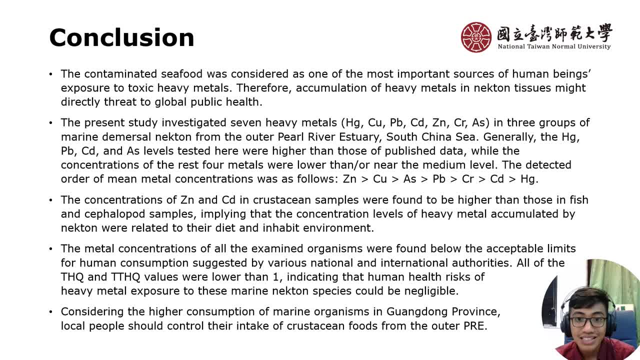 marine nekton species could be negligible. Considering the higher consumption of marine organism in Guangdong province, local people should control their intake of crustacean food from the outer VRE. 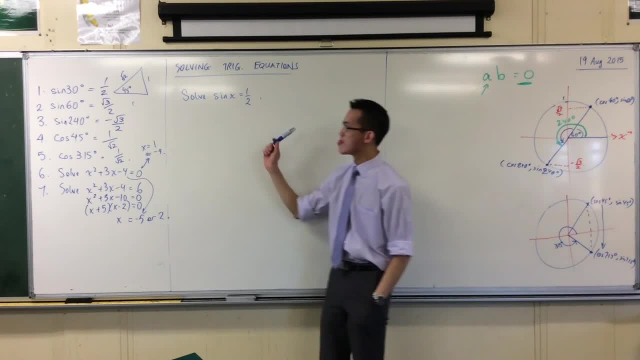 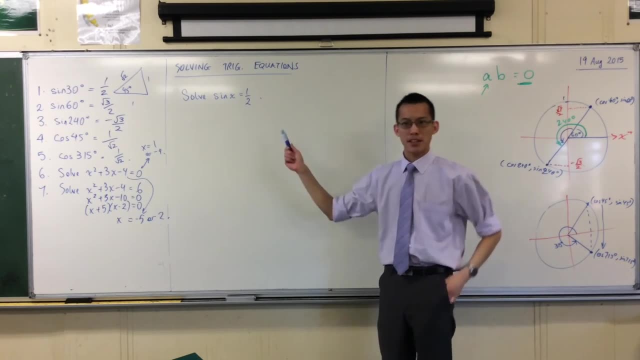 Here's where we're going to begin Now. you'll get these questions a lot, and they appear a lot in two-unit, by the way, So we really want to master this skill. You should be suspicious of this, right? You remember I said I'll often give you questions that will shed light on other questions, right? 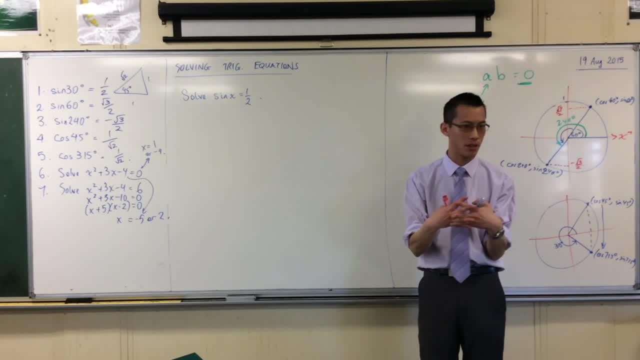 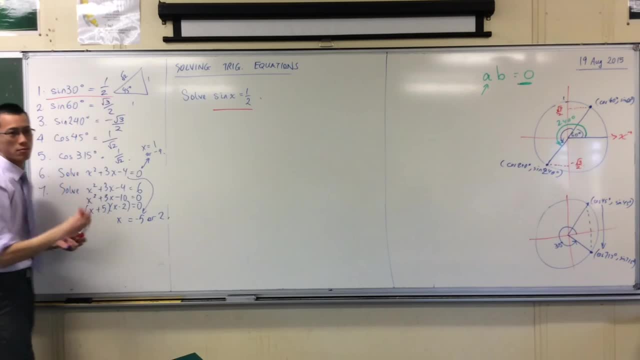 So that you can see the connections between them. Which question on the board is closest to this one? It's just the very first one, right? This guy is more or less identical to this, right? It's just that I popped in a pronoun rule. I've said what's x, Except you already know what x is, right. 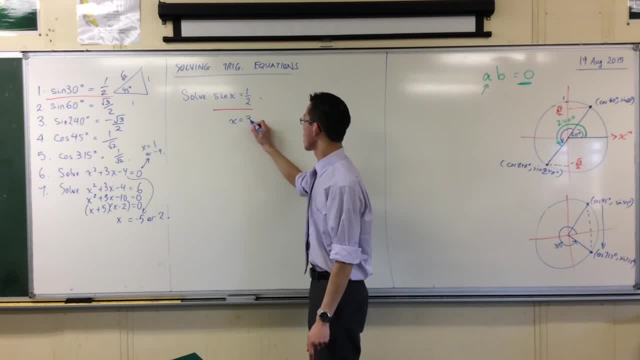 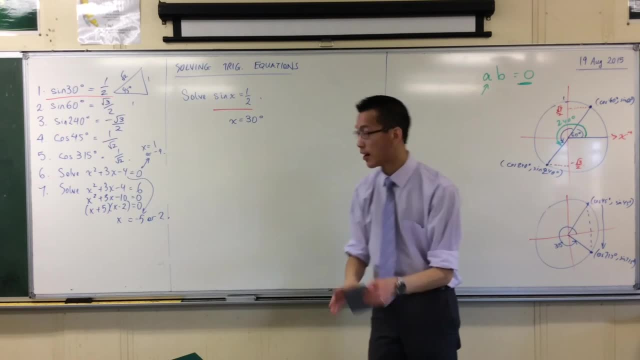 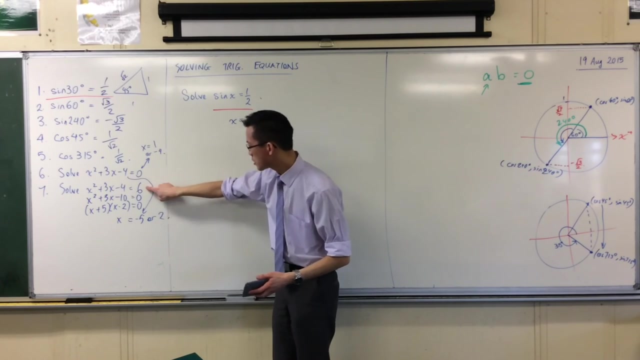 So it's reasonable to say x equals 30 degrees. It certainly worked for us before, didn't it? Now, that's our intuition. You can go to your calculator right, And you can confirm this as well by saying: see how at? let's see this point here. 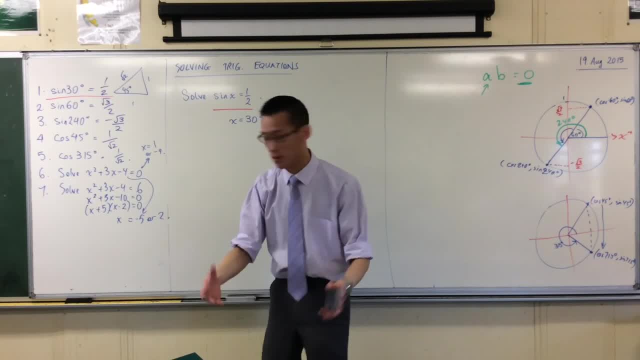 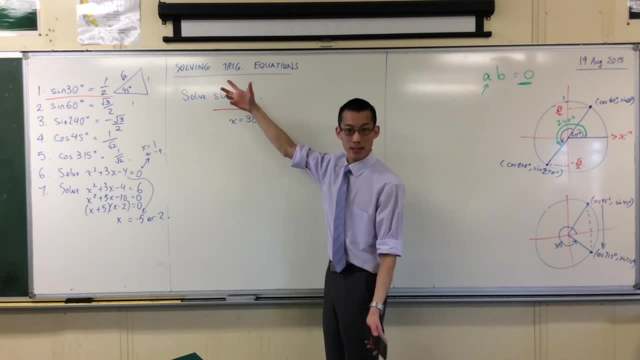 You remember what I'm saying. Do something to both sides. do something to both sides so that you can simplify things, right? Well, What would I do to both sides here to get that x by itself? so it's simpler right. 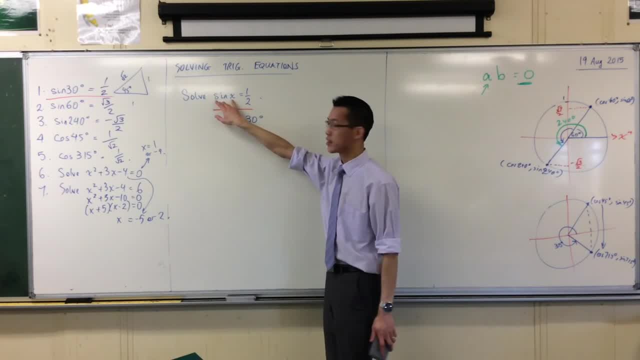 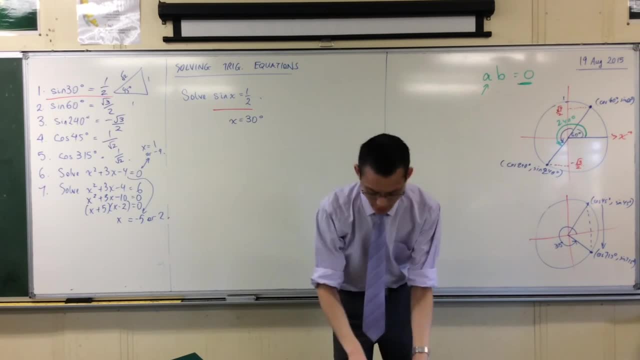 And the answer is: if I want to get rid of sine? you've used this before, even as early as last year. On your calculator, above the sine button, where is it? There it is, You've got this little thing which says: I'll even draw it for you.